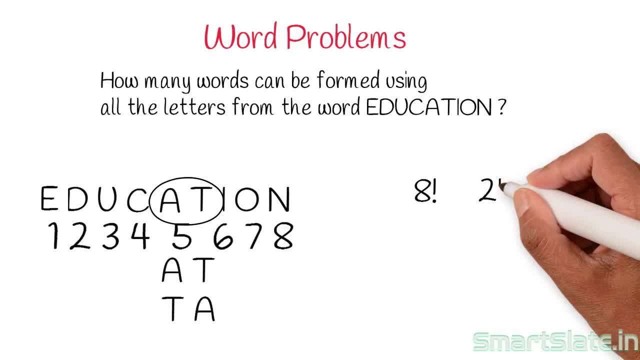 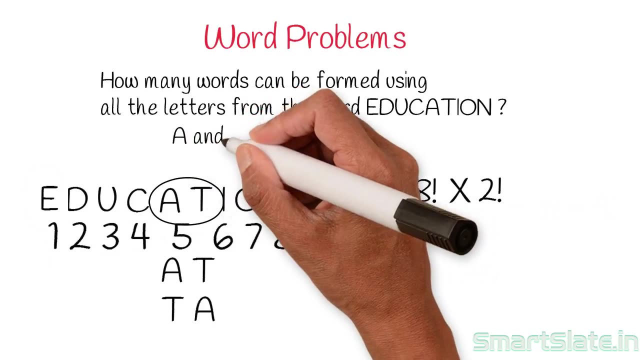 T and T and A, which is 2 factorial. So actual answer to this question is 8 factorial into 2 factorial. I have quickly solved the problem. Next question: What are the possible combinations where A and T are never together? Answer is: 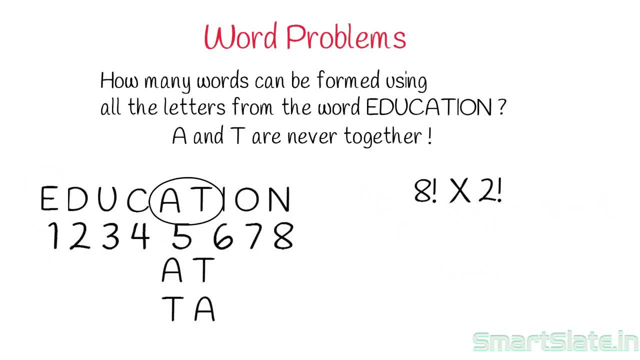 very simple. We know total number of possible permutations is 9 factorial. We also know the number of possible words where A and T are together, which is: 8 factorial into 2 factorial. Substract 8 factorial into 2 factorial. from 9 factorial. You get the answer. 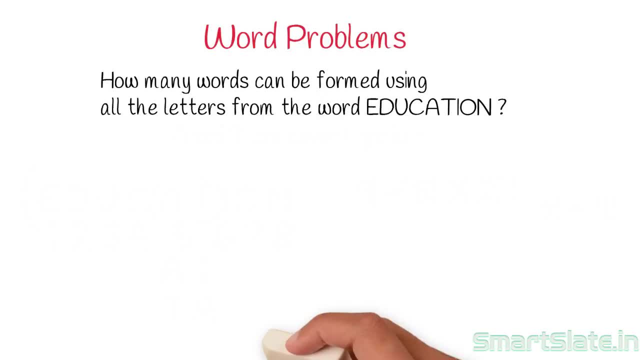 Let's consider some more similar problems. In education, cat should always appear together. The question suggests cat should always be together, not C, A and T, That is, there won't be further arrangements in the word cat, So consider cat as single unit. The number of 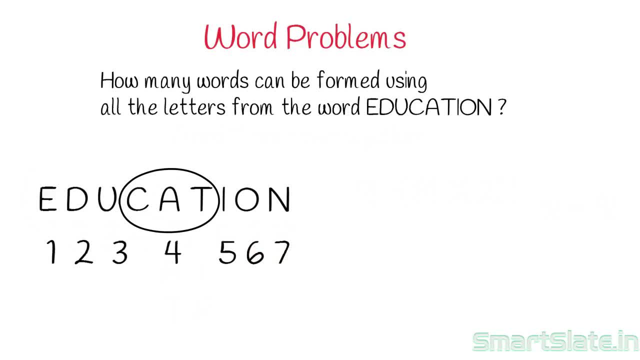 units available for arrangement is 7.. Hence the answer is 7 factorial, Although now the answer is octet. if the quoi nsion says Marc is not included in the size of C, A and T, then the answer should be 7 factorial. into 3 factorial. narstor rico, word qu [ is better, Hence the answer is 7 factorial. If the question says C, A and T should be together, Then the answer is 7 factorial into 3 factorial. I hope by now you are understanding how to solve word problems. Before ending this topic, let me solve. 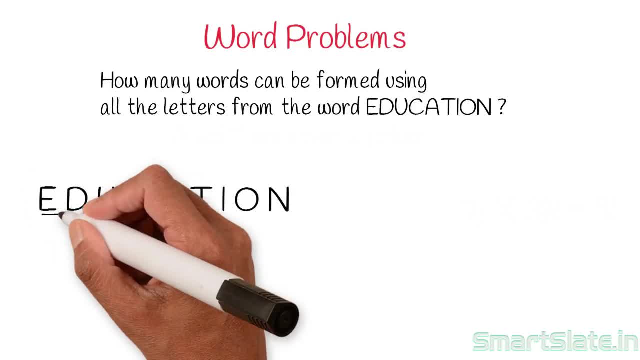 some more word problems. How many words can be formed by letters from the word education, where all three letters are together with the second letter? 2 words too. All the ovals are together. Education has 5 ovals: A, E, I, O and U. 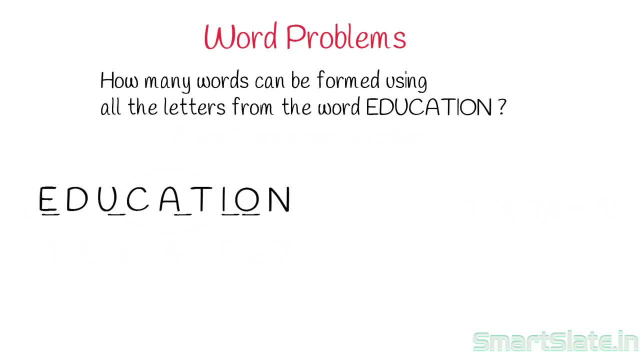 Consider A, E, I, O and U as a single unit, Then possible arrangements are 5 factorial. Since A, E, I O, U also can be arranged in 5 factorial ways, Answer to this question is: 5 factorial into 5 factorial. 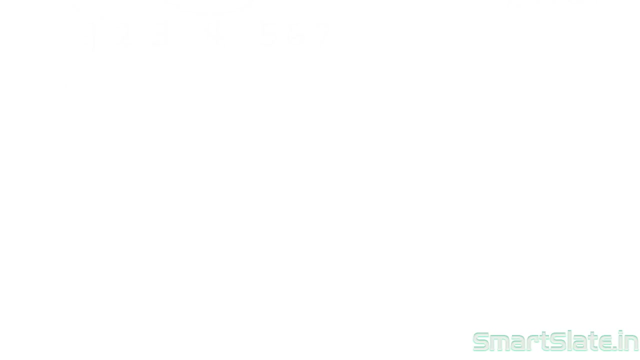 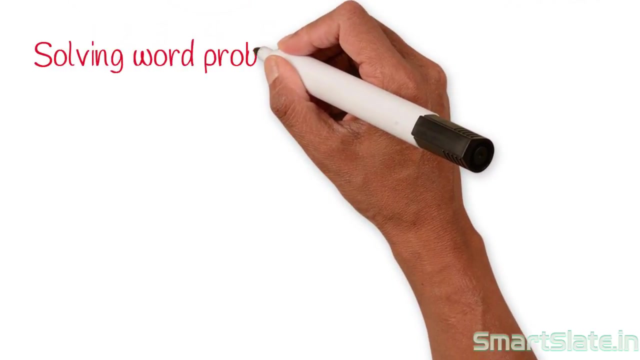 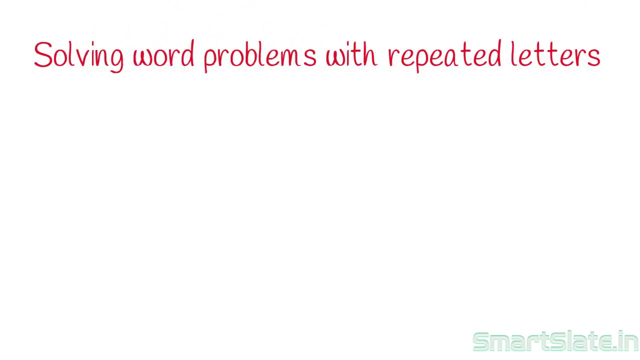 Until now we were using the word education, where letters are not repeated. If the word has repeated letters, then approach to solve such problems is little different. For example, consider a word in I, N, N. The possible arrangements cannot be 3 factorial because N is repeated. 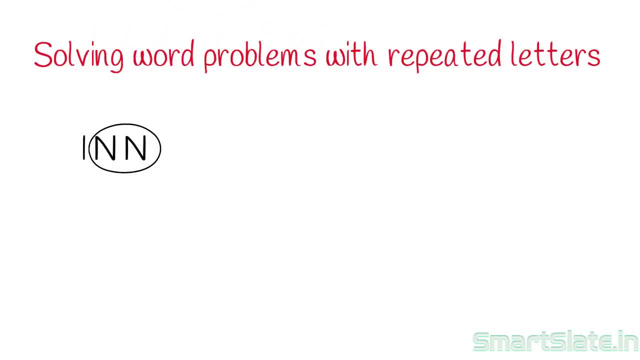 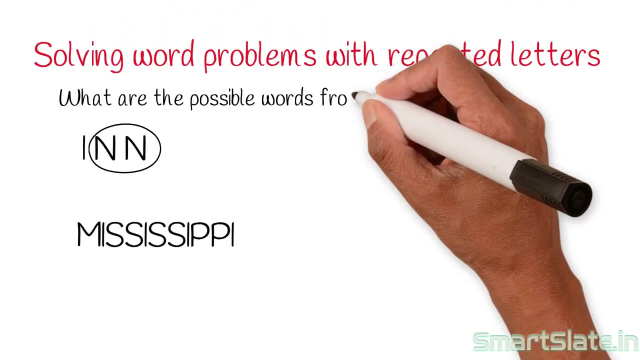 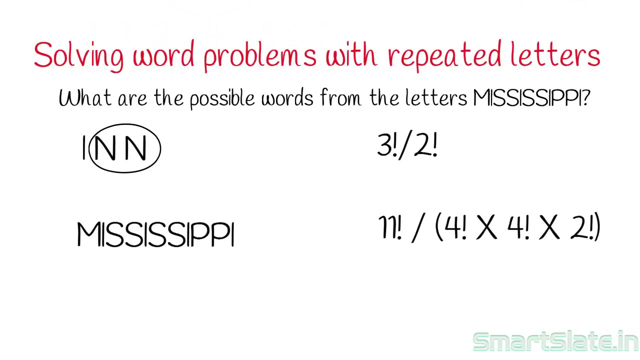 Two N's cannot be arranged. In such cases you always divide permutations of repeated letters. That is 3 factorial over 2 factorial. Consider one more example. What are the possible words formed by the letters from Mississippi? It is 11 factorial over 4 factorial into 4 factorial. 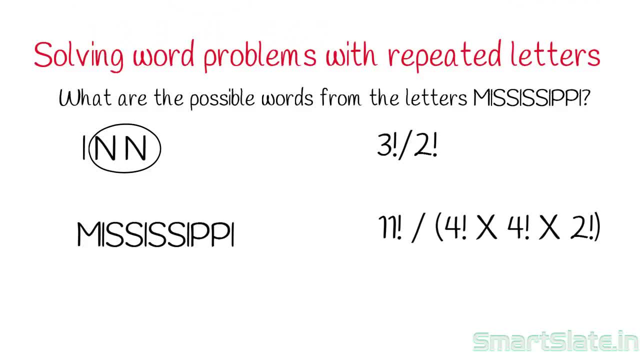 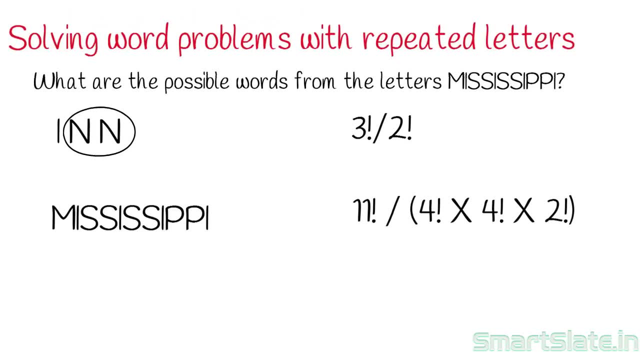 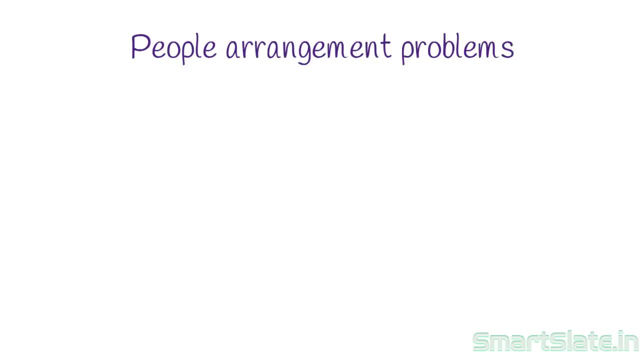 8 factorial over 2 factorial, Because S appears 4 times, I appears 4 times and P appears 2 times. The word problems can be extended to different kinds of problems, For example, in how many ways 8 people can be made to sit in 8 chairs. 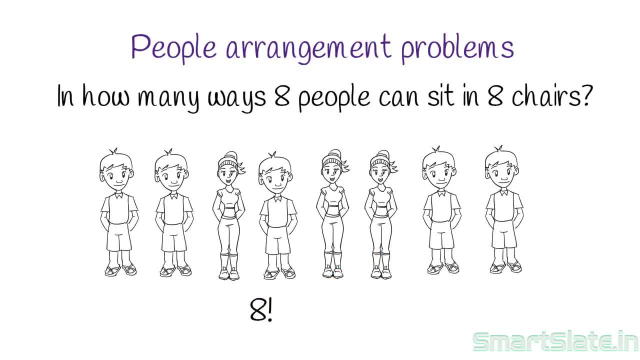 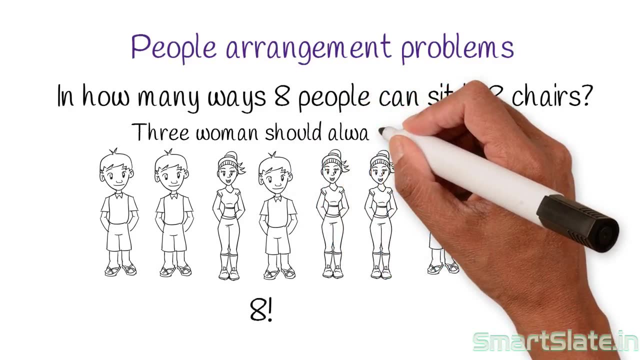 Answer is 8 factorial Treat. each person like a letter From 8 letter words. a word Problem can be still be extended by saying: out of 8 people, 5 are men and 3 are women. People should sit in the chair such that 3 women should always be together, Simple. 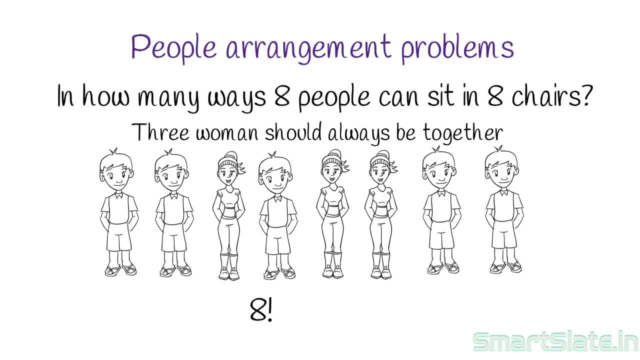 treat 3 women as a single unit or single person. So there are 6 people in total. So 6 factorial arrangements can be done. Note: since 3 women can also sit in 3 factorial different ways, 6 factorial has to be multiplied by 3 factorial to get the answer. So people arrangement related. 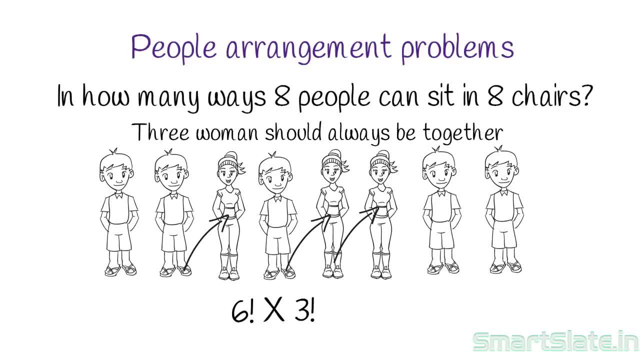 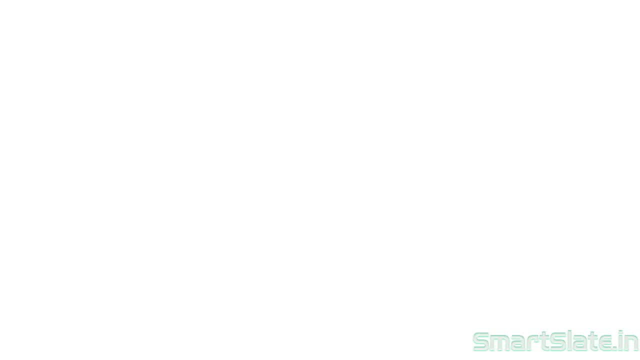 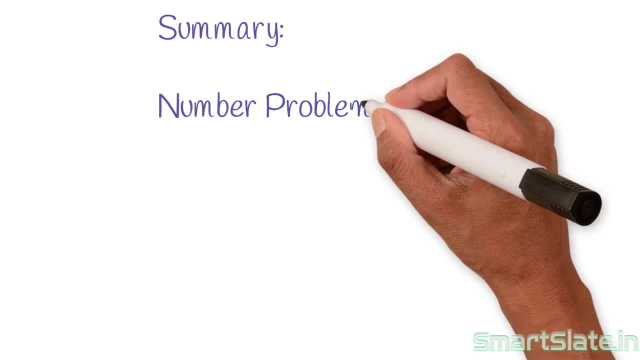 problem can also be solved with the same approach with which we solve word problems. Whenever you get permutation and combination related problems, try to break it down and make it as simple as possible. I have explained some niche topics in permutations and combinations, such as number problems.